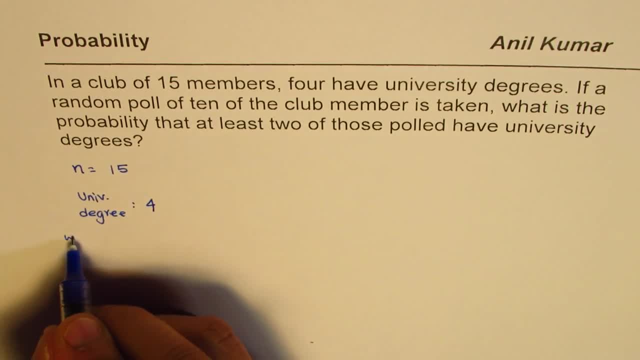 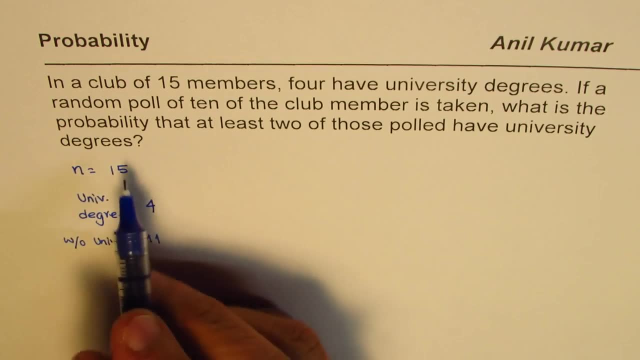 is with 4.. That means without university degree. we have 11, right. So that is how this happens. distribution is if a random poll of 10 of the club members is taken, so are the value which we are taking is 10, what is the probability that at least two of 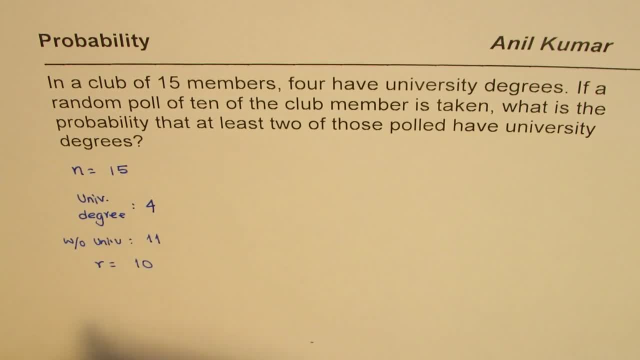 those poll are with university degrees, so we are looking for probability where the random variable will be at least two of those polls is having university degree. that means two or more should be having right, so X value should be greater than. I should actually write greater than or equal to two right, so at 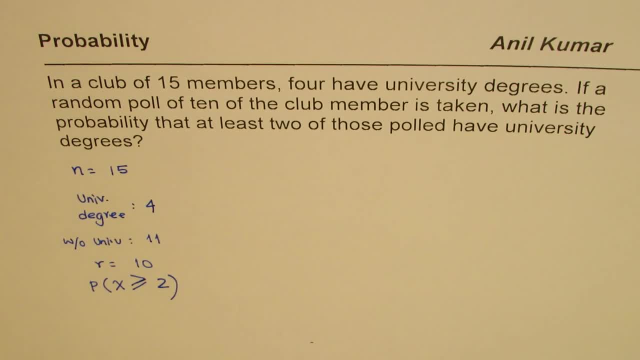 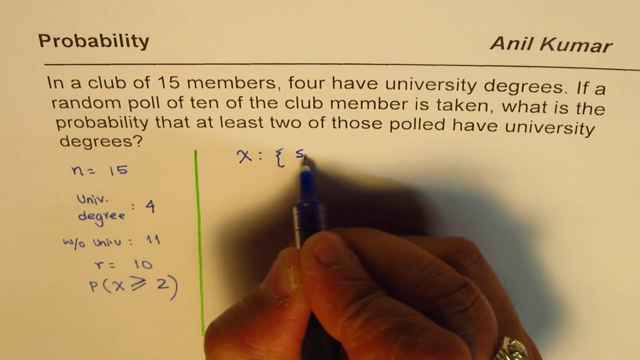 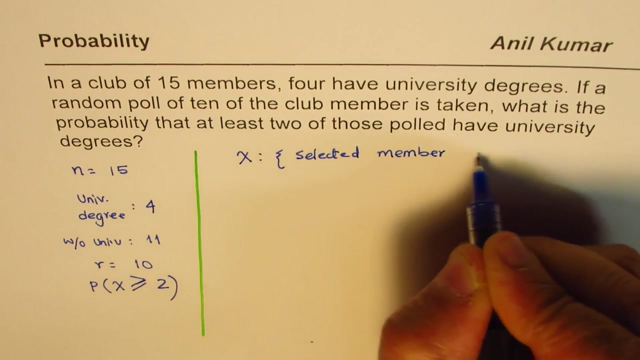 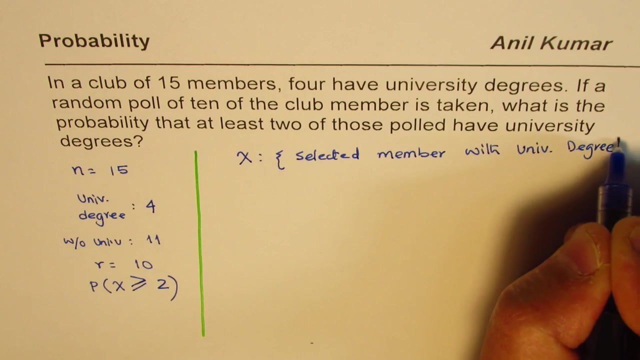 least that is what it is now. here we have defined the random variable as the selected member having a university right. so in our case we are defining random variable as selected or poll member with university degree. is it okay? so that is how we've defined it. now, when we say that the probability is greater than 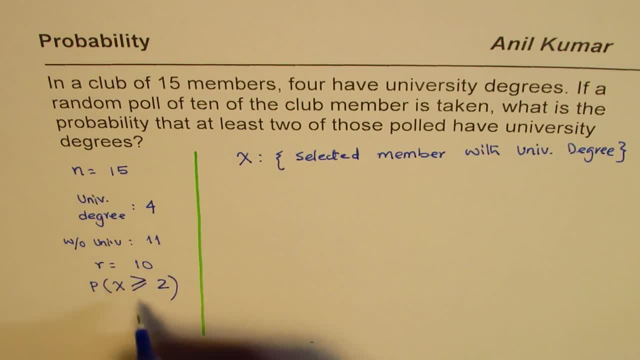 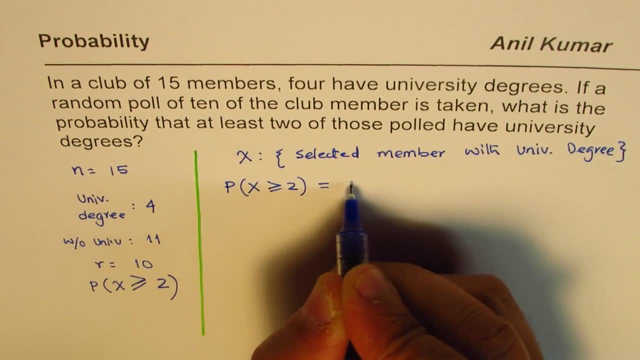 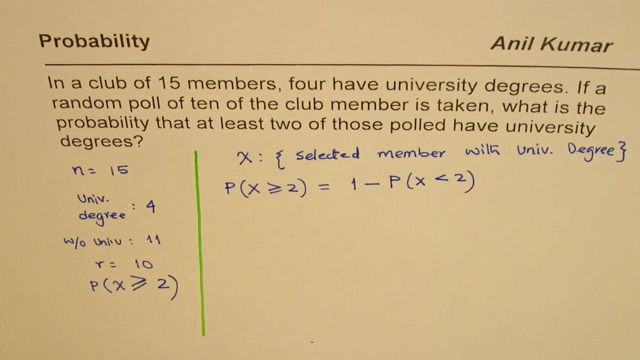 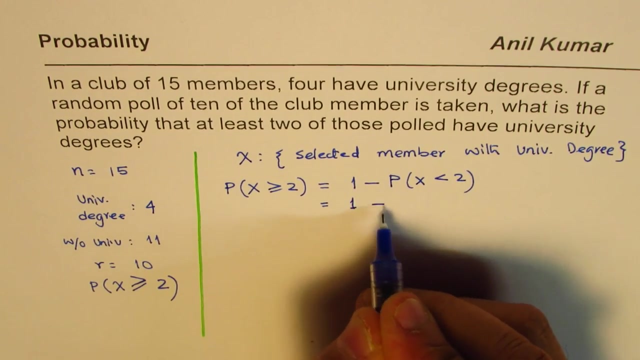 equal to two, total probability is one, so so we can actually get like this: probability for X greater than equals to 2 will be to 1, minus probability for x less than 2, is it okay? so so that makes things a bit simpler for us- which could be equal to 1 minus probability when none of them has university degree. that 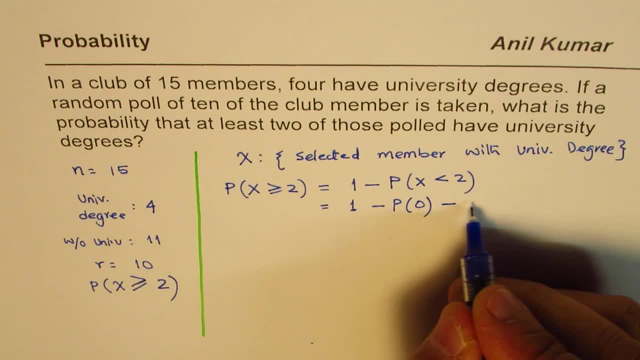 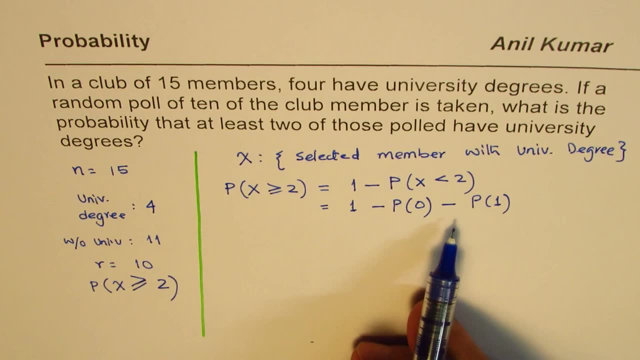 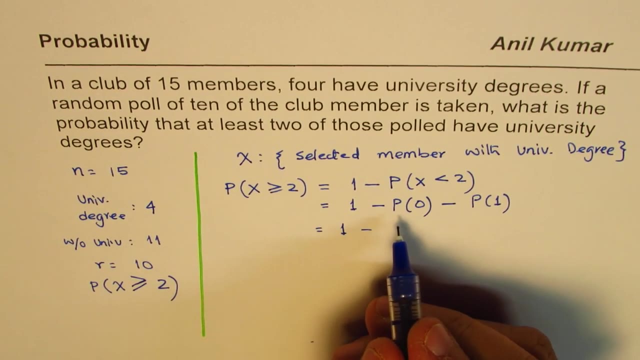 could be one case, or the second case will be when x equals to 1, so let me write this as probability: when 1 has university degree, is it okay? so that is how we can think about right now in this case, none of them having university degree. there are four with university degrees. we are selecting. 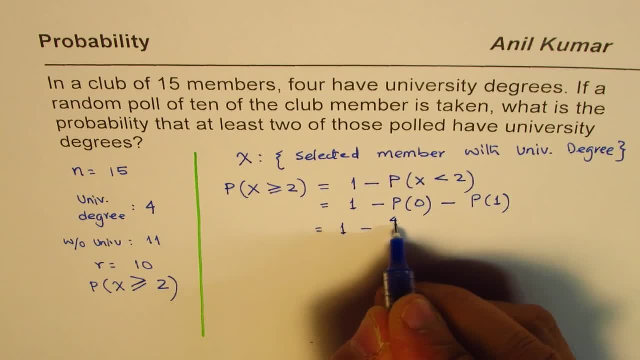 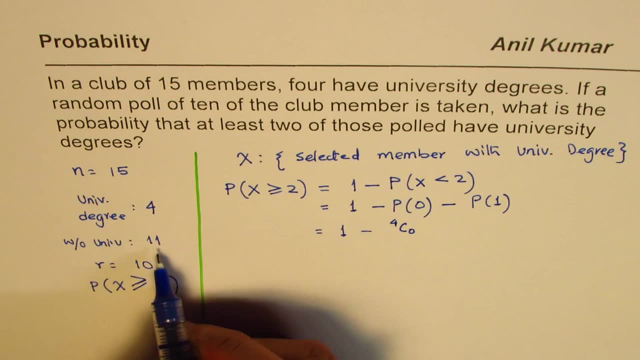 none of them right. therefore, that should be 4 C 0. so that means all which have been selected are without university degree, right, and we are selecting how many ten of them, correct? So all 10 selected are without university degree. So it will be out of 11, 10 will be selected without university degree. 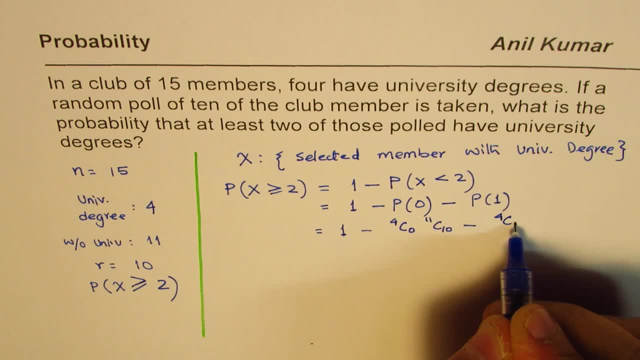 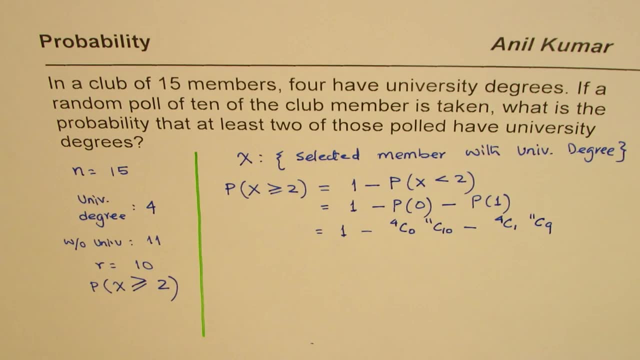 If you select 1 with university degree, then it becomes 4C1 and that becomes 11C9 will be selected. So these are the selections, and total number of combinations for each are how many. The selections are being made from a group which has 15 members and we are selecting 10, right. 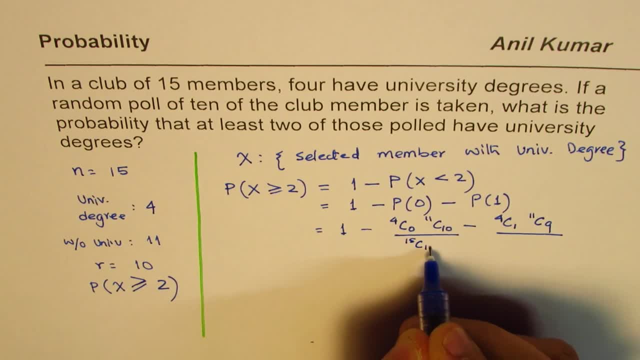 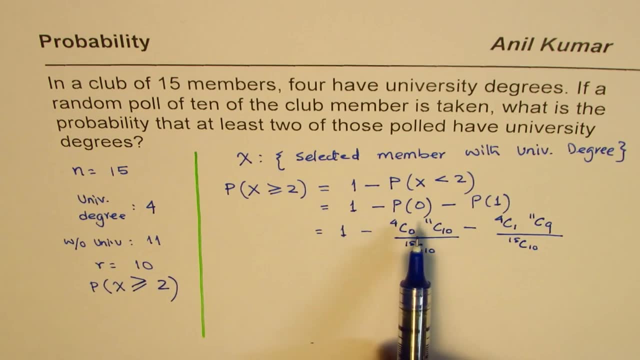 So therefore, they should be divided by 15C10,, is it okay? So that is the probability. So the probability for none of the member with university degree is 4C0 times 11C10 divided by 15C10. 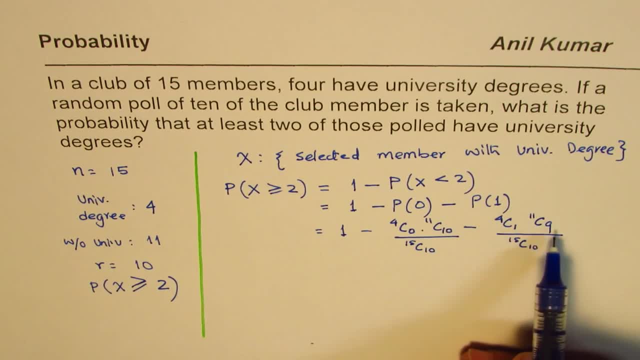 And the So 1 with 1 degree will be 4C1, 11C9 divided by 15C10.. So that is your answer, right? So now you can actually calculate these values using a calculator and then find the answer. 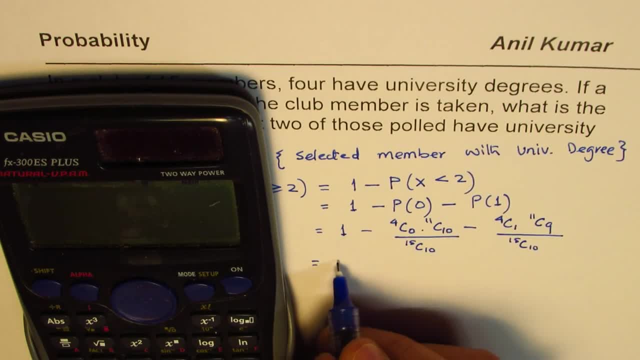 So we have 4C0, so it is 1 minus. 4C0 means 1, right? 11C10 means it is 11, correct? So let's calculate what is 15C10.. So it is 11 over 15C10, right. 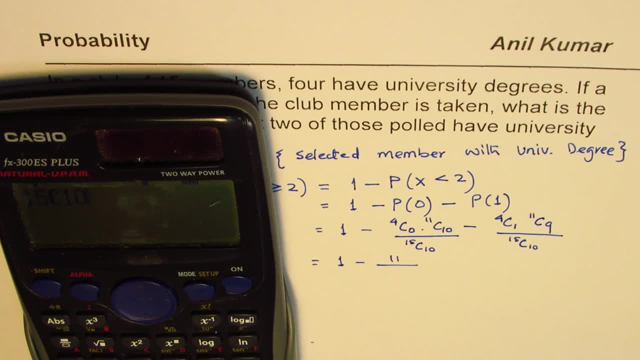 So 15C10,, which is equal to 3003, right 3003, correct Minus. So now we have this term 4C1, which is 4.. Anyway, let's Okay, so it is 4.. 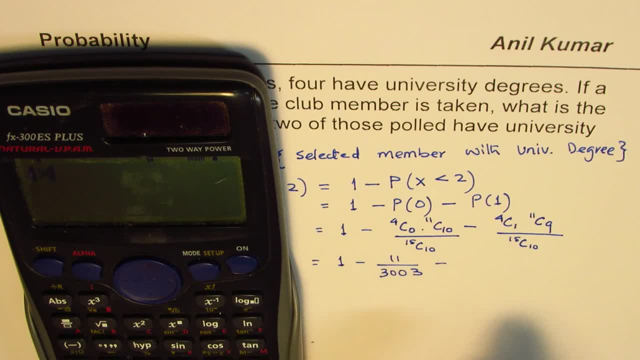 4 times. Let's do 4 times 11C. Let's calculate this value: 11C, C9, which is equal to 220.. So we get this as 220 divided by 15C10.. We calculated 3003, correct.